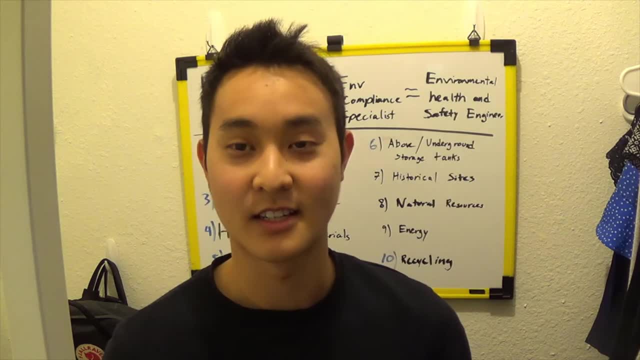 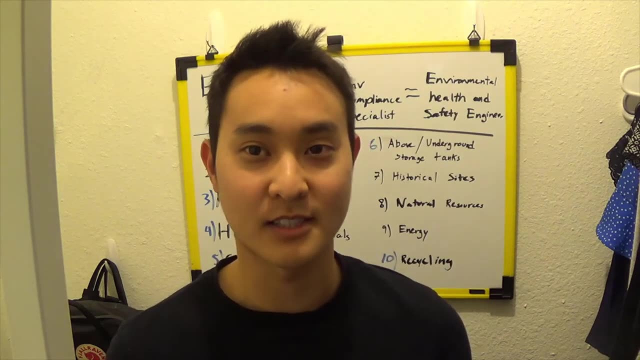 engineers do and it gives out a pretty broad definition. They say something like they do engineering practices that helps the environment or pollute less. They try to make processes more efficient using engineering practices and so on. Just something very broad and general like that. 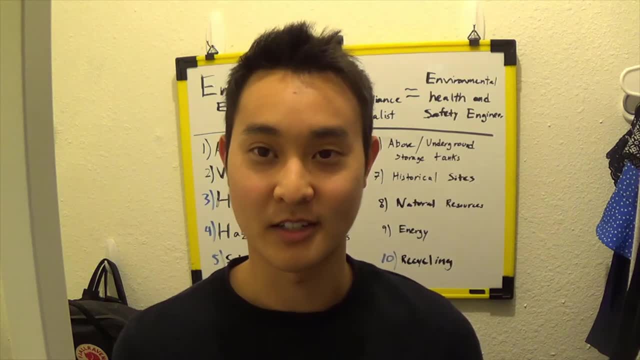 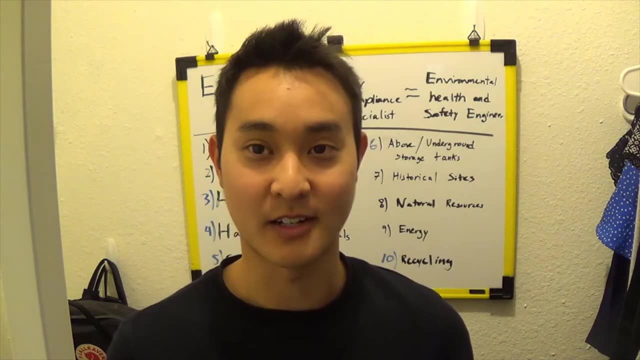 But that to me is very broad and doesn't really help distinguish what every environmental engineer would be doing. And sometimes you go to school you'll be learning one aspect of a field, but then when you go out and find a real job you don't use any of that thing that you learn in school. 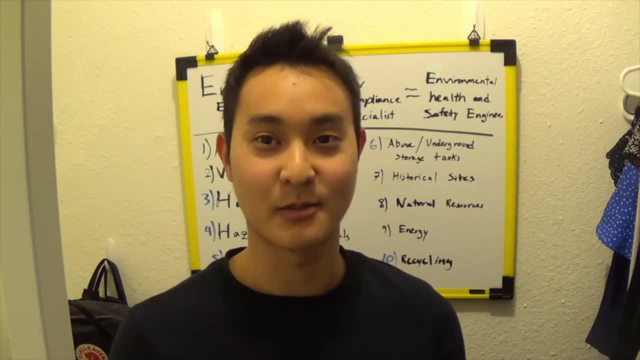 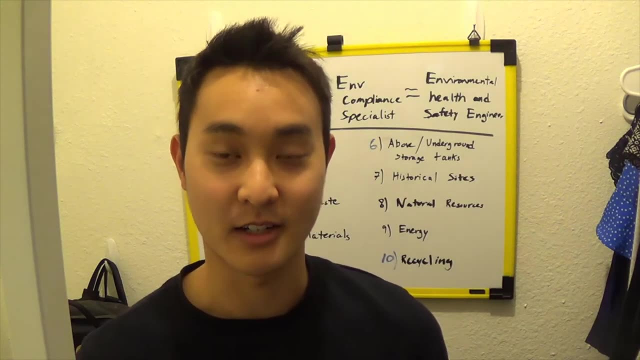 So in this video I want to tell you straight up that probably what you learn in school won't be what you're going to be doing on a job. So currently I have the title as an environmental engineer at my work, But when I google what environmental engineers do, I notice that some other job titles have the same job. 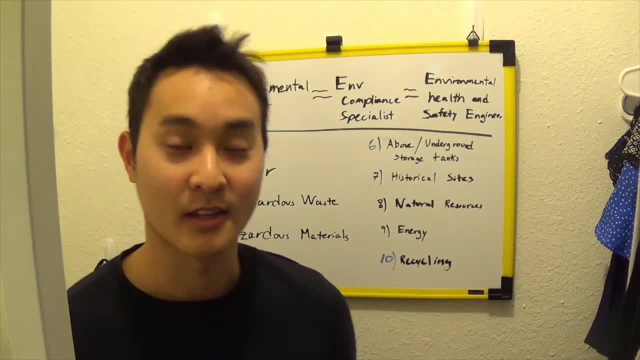 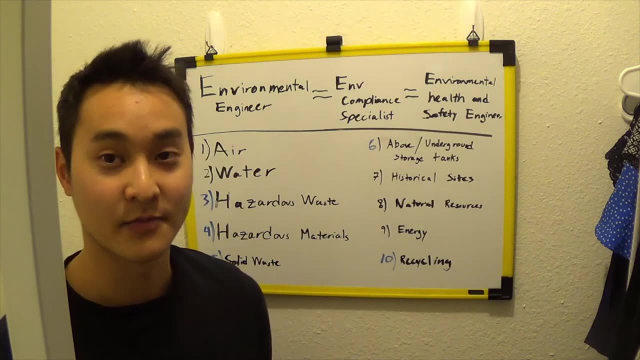 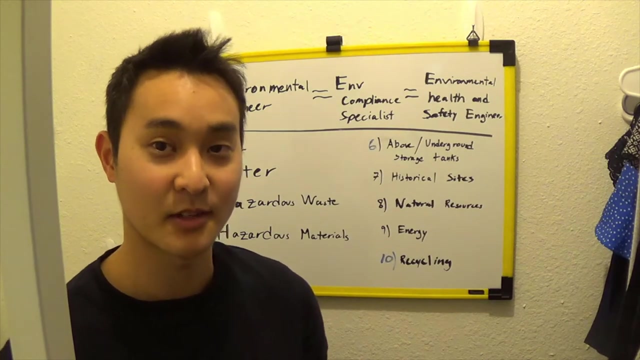 description. So my job description is an environmental engineer and hopefully you guys can read this. I'll just get my little pointy stick. I'm an environmental engineer here, but when I'm looking up online, I noticed that an environmental compliance specialist does the same thing as to what I'm doing right now. So in a way, even though I have the title as an 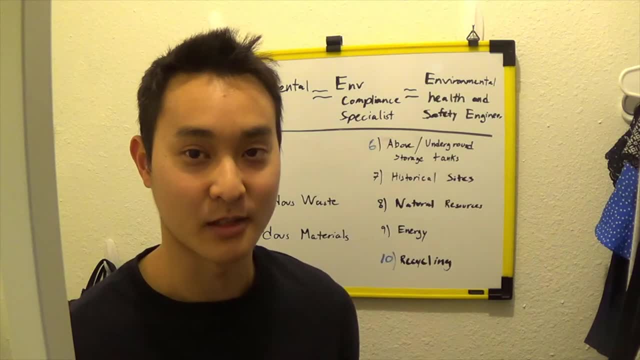 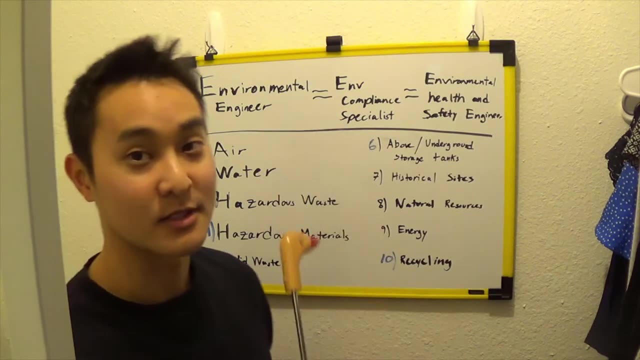 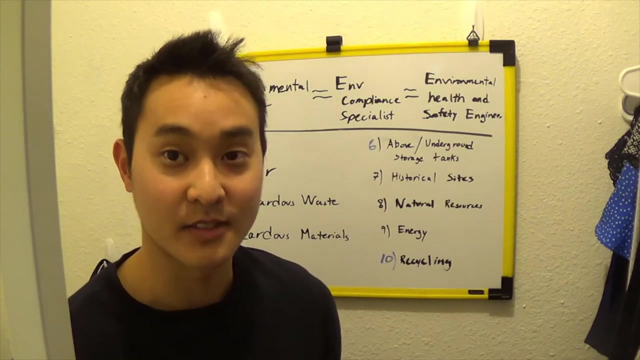 environmental engineer. I can pretty much interchangeably say that I'm also an environmental compliance specialist. So I've seen job descriptions that have environmental compliance specialists with the same job description. I've seen environmental, health and safety engineers with the same job description. again, We're doing the same thing. it's just that we have different titles. So this is why. 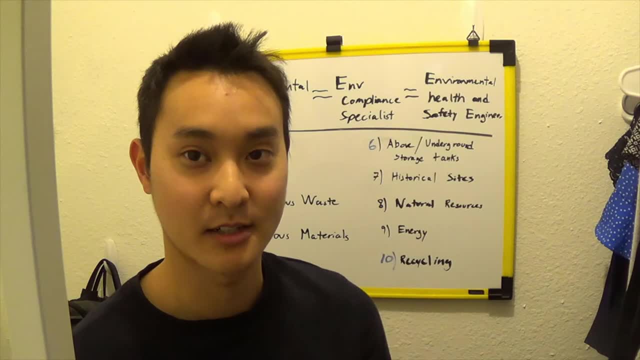 I want to clarify that. you may have the title as being an environmental engineer, but you might be doing something similar to that of an environmental compliance specialist or an environmental safety engineer. Okay, so I just want to point that out. They might have different pays. They might have different job. 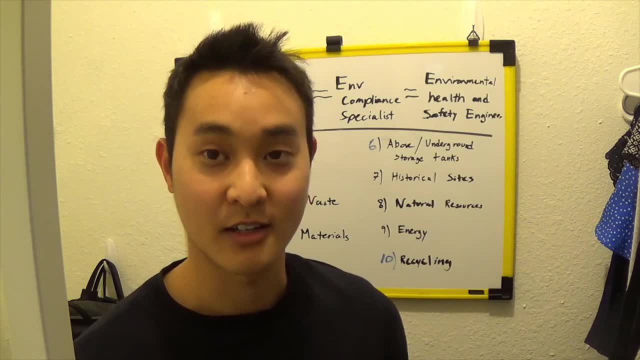 requirements and certifications, But overall, you guys might be doing the same thing and working together, side by side with your whatever job you're doing. Okay, so now on to the juicy part. So here's what I do at my facility. In each job, each environmental engineer will be different, So 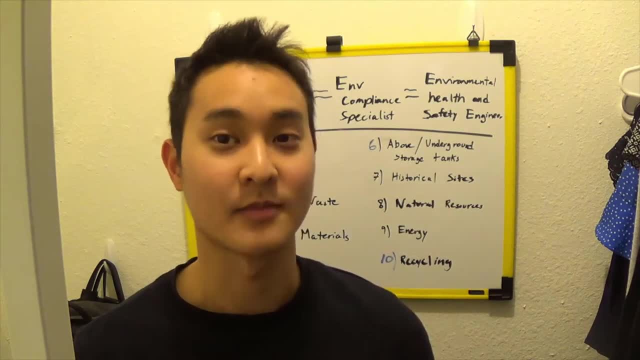 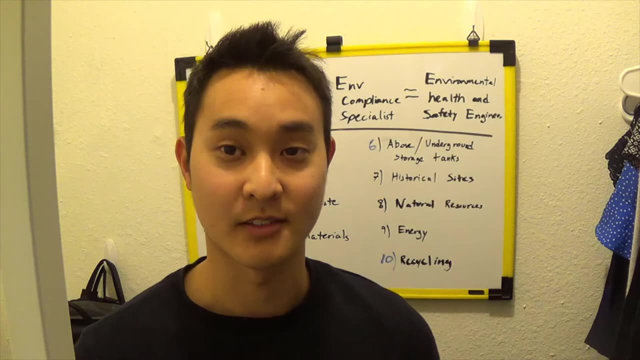 at my facility. you can imagine it as being like a little city. I'm just going to be pretty straight forward. I work in an air force base, So in that air force base there's things like the commissary, So that's where they. 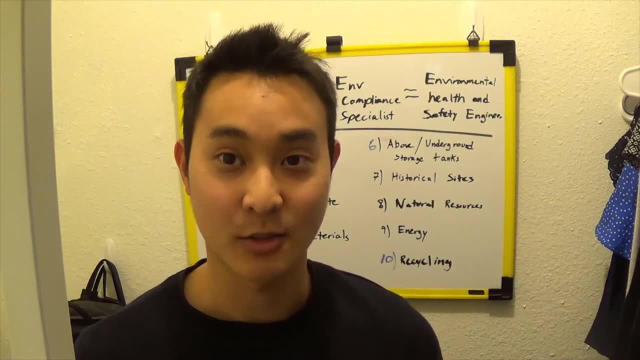 process foods. They have a gas station, So that's where they have like storage tanks, You know gas tanks. They have a medical clinic. They have a dental clinic, So they have things like you know, pharmaceuticals and maybe dental cleaning supplies. They have maintenance operation vehicles, So you 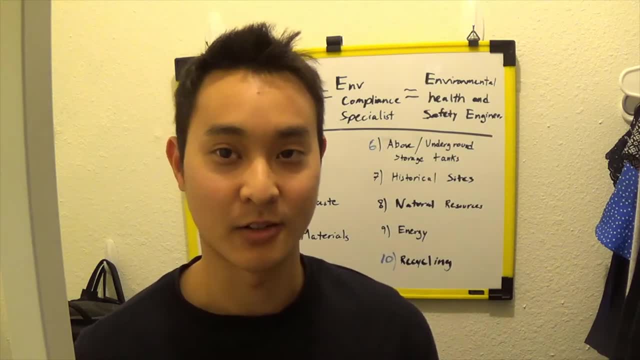 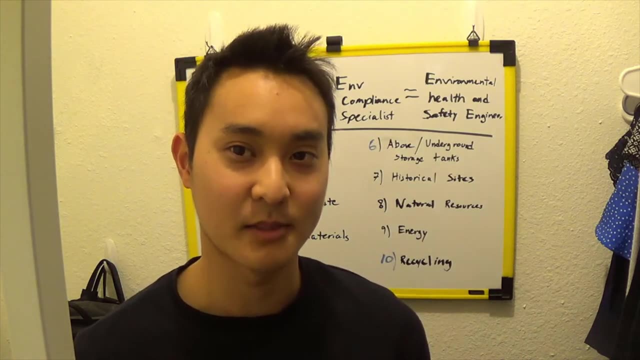 know people who are cutting the grass. they have to put it in like the gasoline, their oils and so on. We generate waste too, So we have things like trash. You have recyclables And so on. So, again, just like a mini city, you have to monitor different things within this facility. 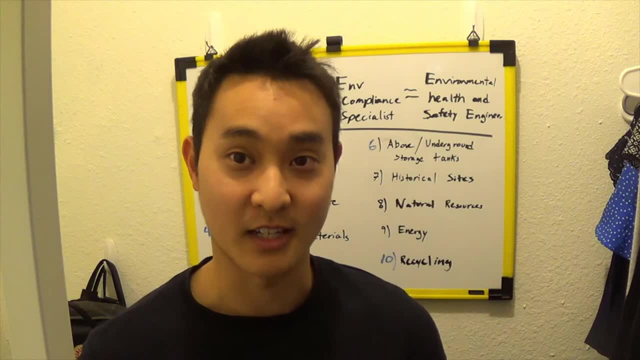 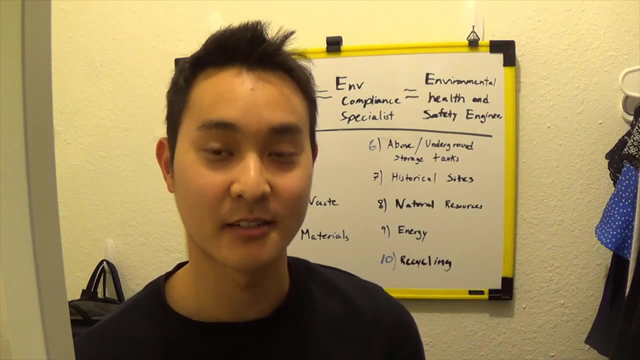 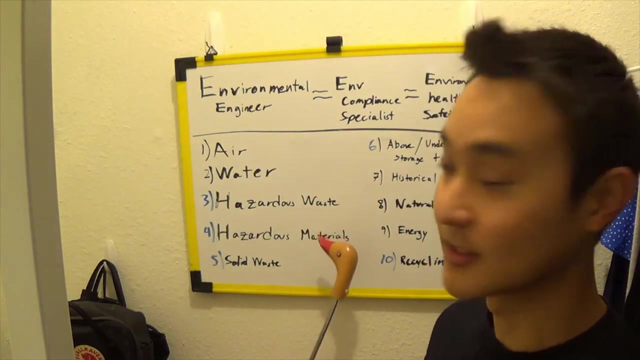 And so that means we have different programs that we have to allocate with each environmental engineer at my work, And behind me is a list of some of the categories I can think of. So some of the environmental programs that we have is things like air, water, hazardous waste, hazardous materials, 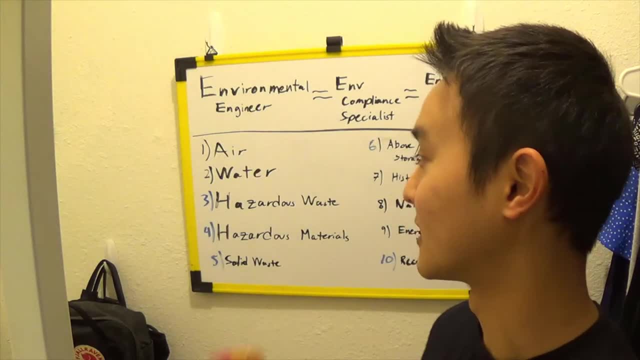 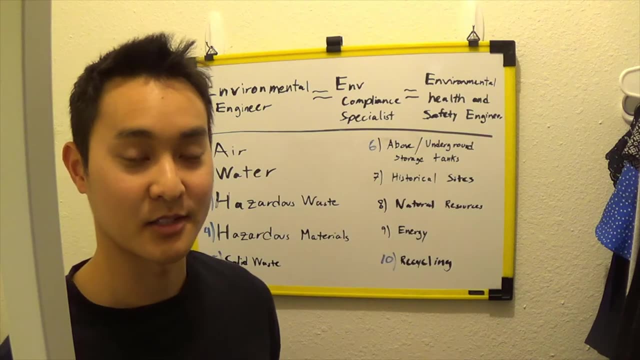 solid waste Again. you can just imagine this as a mini city. So we have things that you have to monitor: underground storage tanks. this is the gas station. we do have some historical sites, because we still have to monitor and make sure that we're not like digging up any fossils or anything. if we're trying. 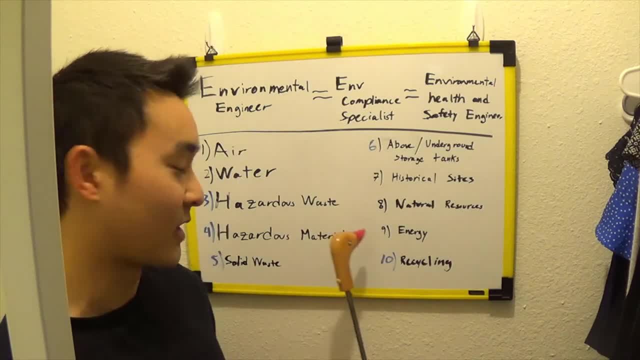 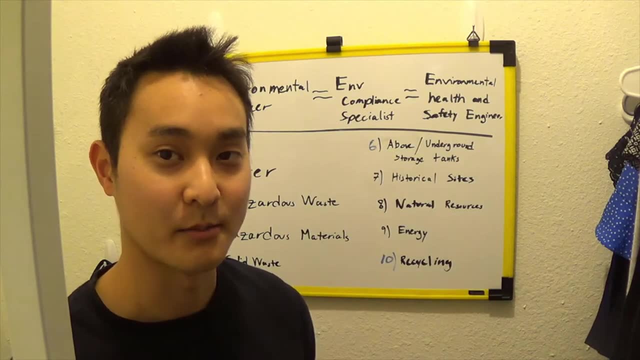 to do some construction projects. you have natural resources, energy and recycling and so on. this is just a list of a few things that i can think of currently at the top of my head, but i'm pretty sure we do have more. i just don't know everything all together right now, and so we have all these. 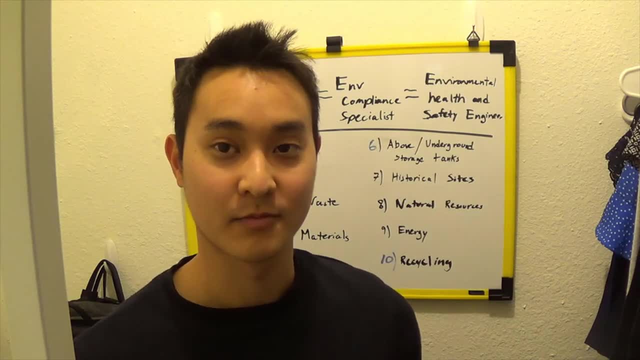 programs that we have to monitor and make sure that we're following, because we have federal rules that we have to make sure that we're following. so epa sets these rules and because we're living in california, we have even more strict laws. so overall, each state will have certain laws that 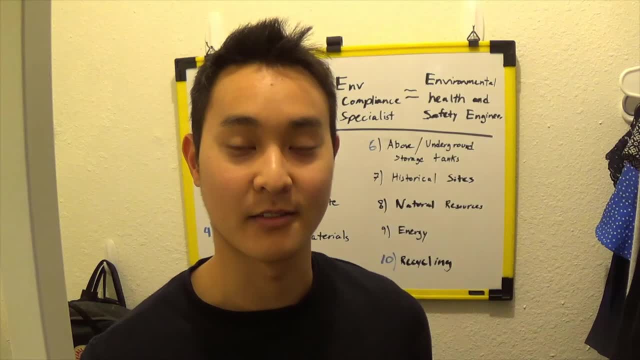 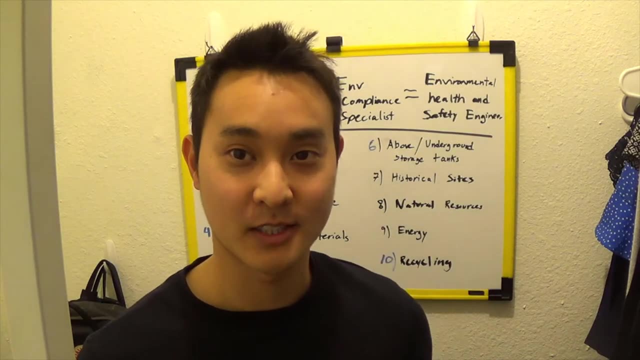 they'll abide by, and california, being the most strict, will probably have more strict rules, meaning you're not allowed to pollute even more than the federal laws. i hope that concept wasn't too confusing for you to grasp. so let's go back to these environmental programs i have on the board. 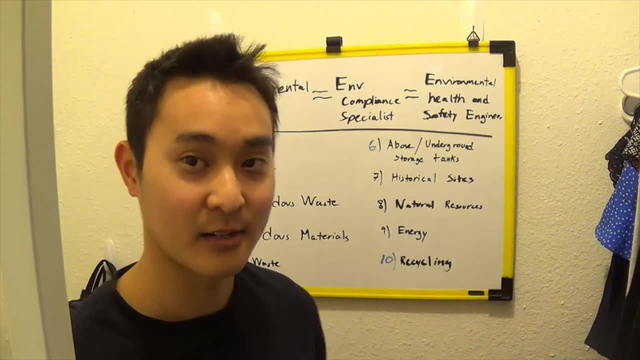 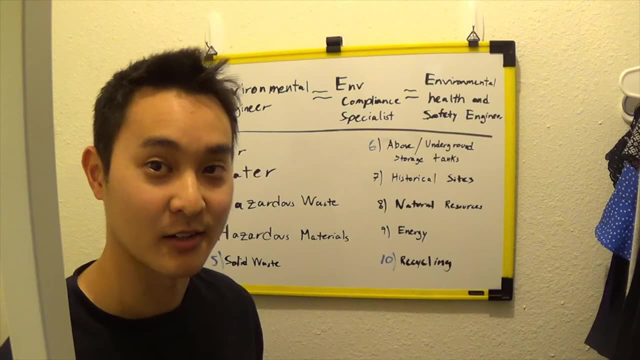 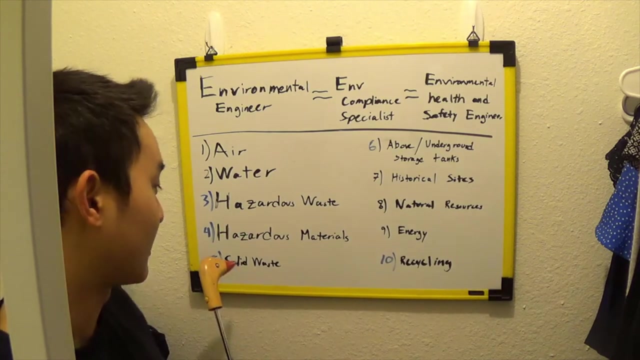 so i have a list of 10 environmental programs here, but i don't manage all of them. this is split up between all of my co-workers, so the ones in blue are the ones that i currently operate and manage. so i operate and manage hazardous waste, hazardous materials, solid waste, recycling and 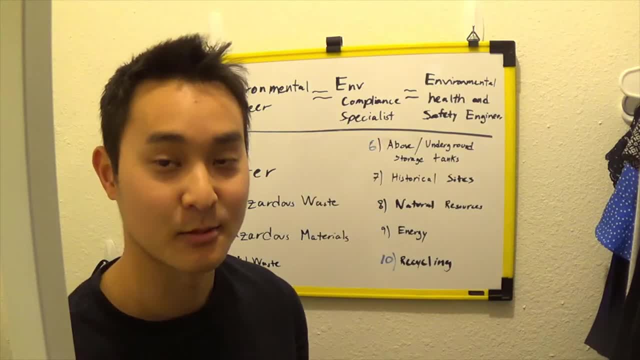 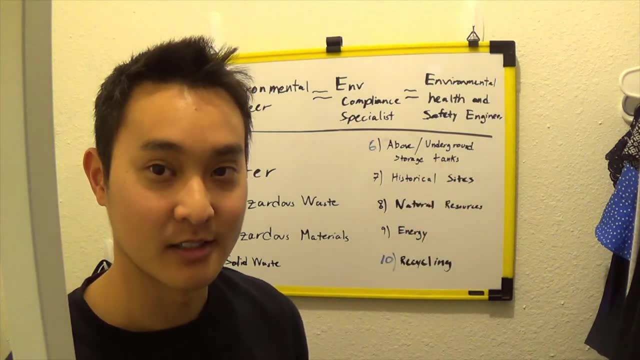 some of the above and underground storage tanks. when my co-workers in there i'm just trying to like just touch the water on that. so i'm not too familiar with that program, but i am starting to delve into that, just in case he happens to be sick or is on vacation. 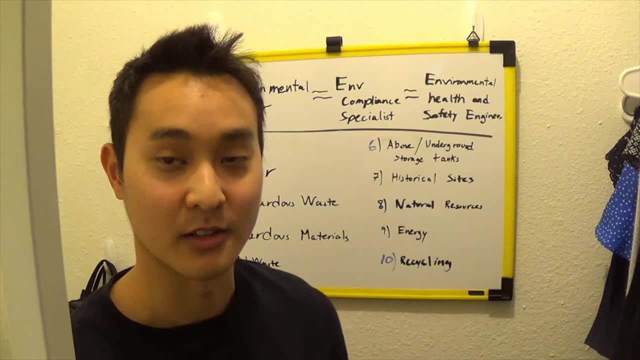 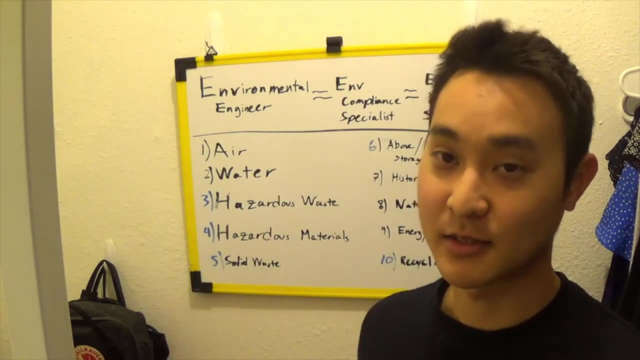 I can at least answer some questions on this program, Although, again, I'm not the specialist in that program. So let's go over hazardous waste and hazardous materials. Really, that's my specialty at work. That's what I do mostly on a day to day basis. 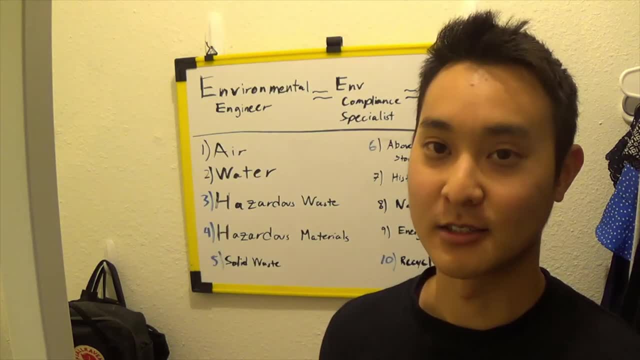 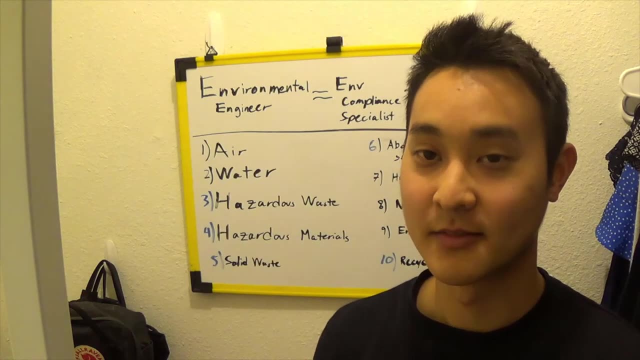 So what does this mean when I'm in charge of this hazardous waste, hazardous materials program? So, going back to my facility, we have like a maintenance crew that uses oils and produce all the rags. They have gasoline in their vehicles. The whole point of this hazardous materials program is to tell the air force. 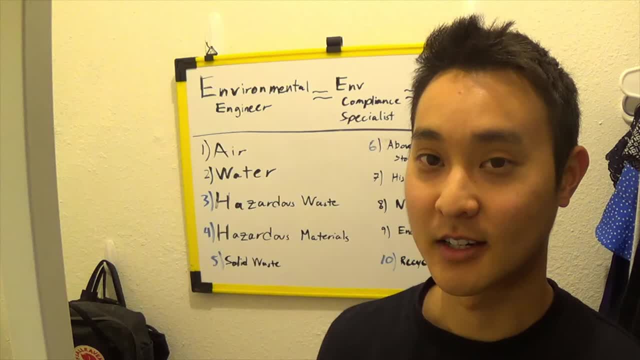 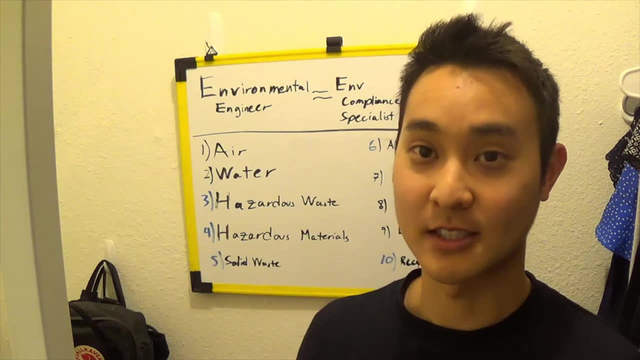 saying: Hey, these guys, this operation crew, they're using, say, 500 gallons of oil every single month, And so we just have to make sure that the air force is informed as to how much a certain material is being used and how often they use it. 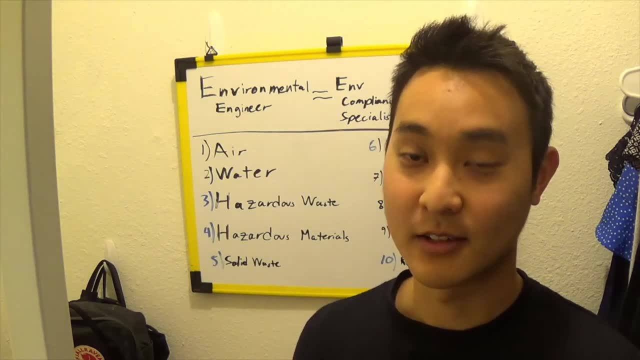 Overall, it's just trying to make sure that they know what we're using. They want to know that. we know that it's dangerous And overall it's just to inform everyone that we are using this material and this much amount. We're here to monitor and make sure that everyone is following the rules and 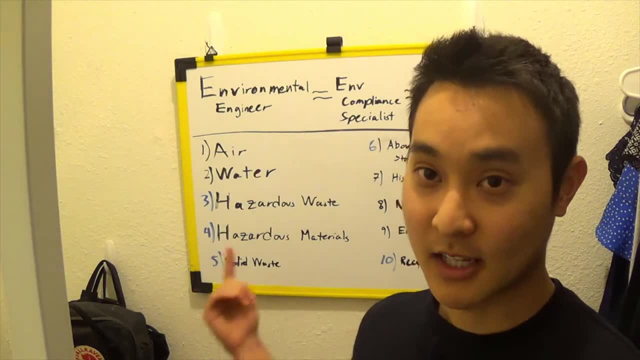 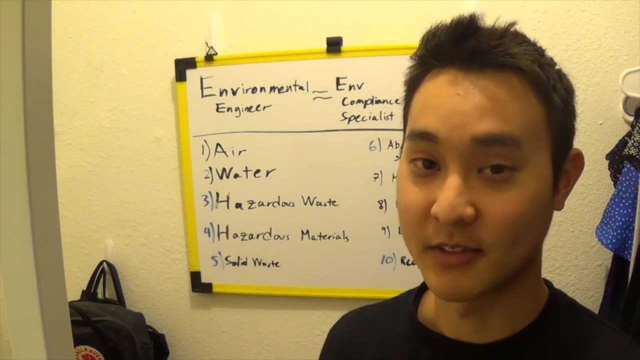 that we know what materials is on base and how. I monitor this hazardous materials program is really. I'm just walking around the base inspecting, saying: what do you have? What are you hiding? Do you have everything stored properly? Do you have everything labeled? 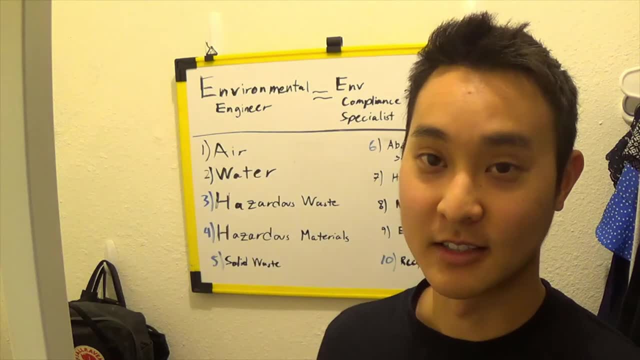 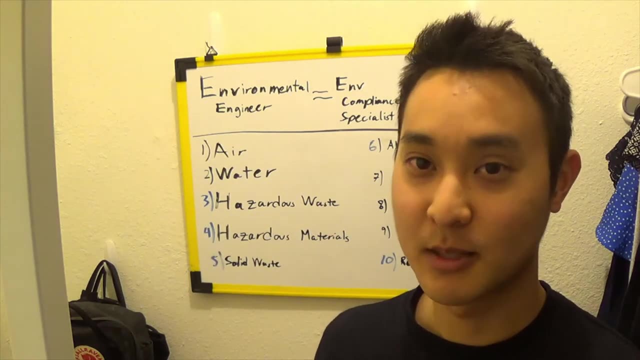 So if I open this bottle here, will I know what's inside of it, You know? is it poisonous for me or is it just water? How much of it do you have? How often do you use it? I'm really just talking to people to make sure that they're following the rules. 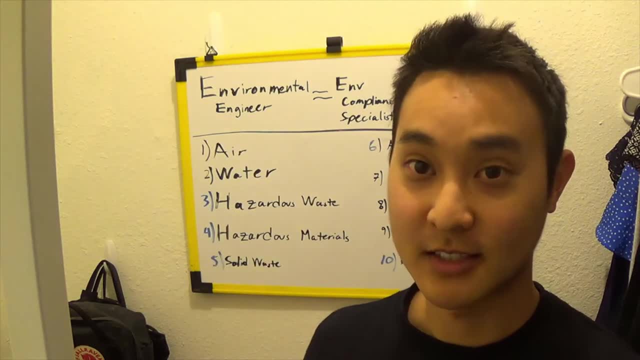 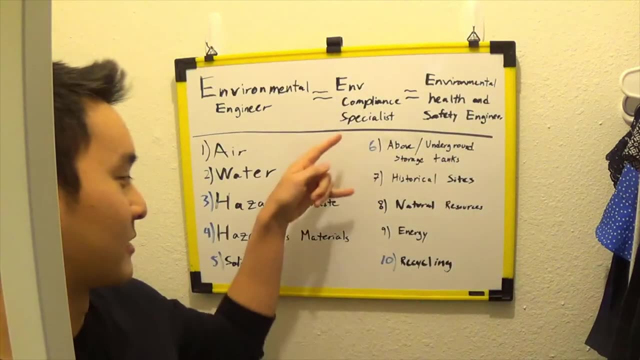 making sure that it's labeled and stored properly, And so that's just one of the environmental programs that I'm dealing with. That's just how I handle hazardous materials. I don't really want to go over all of it. I know I have some other blue things here on the list. 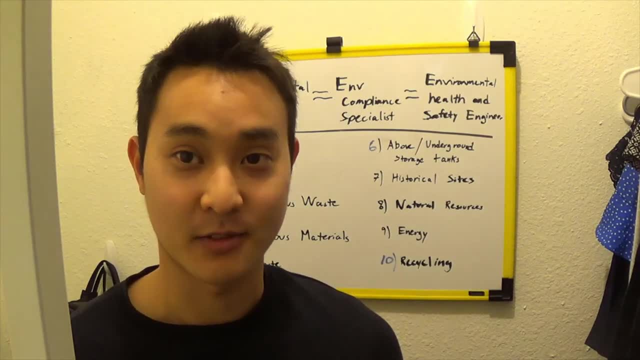 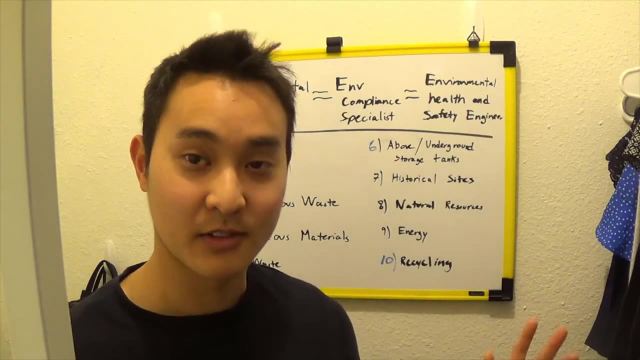 but that's just sort of a bit too much for you to take on as of right now. Maybe in the future I'll go over into more detail as to what I do on a day to day basis, But overall I just want to give you the gist as to what environmental engineers do.